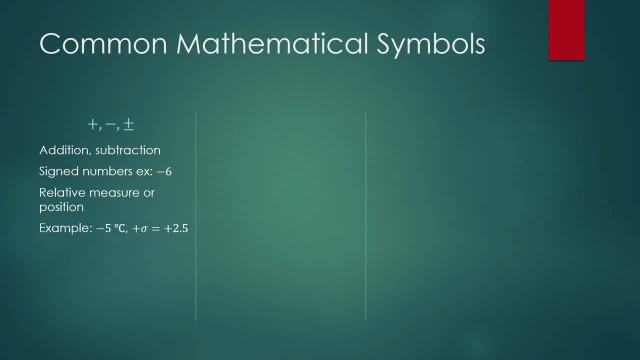 Sometimes it only comes round one, sometimes it comes round five. We'll read the data again. You're always having situations of sharpening off the edges, with the model being too huge. the mean that means your score is somewhere between 8 or maybe better than. 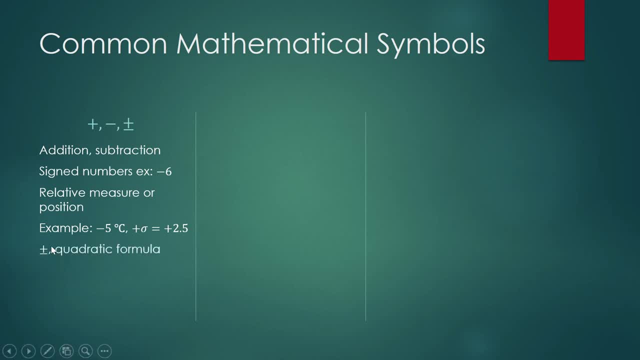 8.5 to 9.. We saw this symbol- plus or minus- in the quadratic formula. What is the meaning of this? The meaning of this is: X would have at least two values. The first value is negative b plus the square root of that, all over 2a, and the 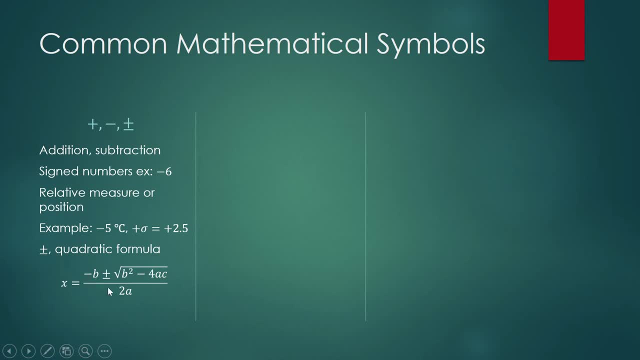 other value is going to be negative: b minus square root, all over 2a. Plus or minus also means adding a margin of error, So sometimes you will see something like this: This is the symbol for average or the sample mean. So the sample mean is, let's say, for example, 65 millimeters plus or minus 3 millimeters. 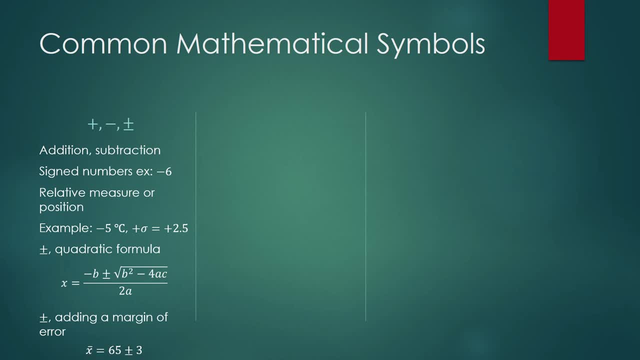 So that means the average measurement is not exactly 65 millimeters. It's somewhere between. Okay, So it's going to be somewhere between 62 millimeters and 68 millimeters. 62 because 65-3 is 62.. 65 plus 3 is 68.. These are our symbols for. 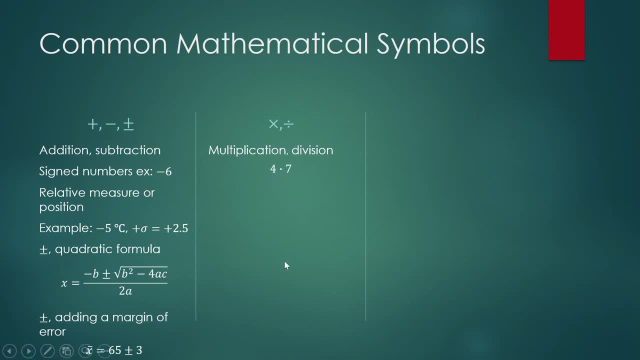 multiplication and division. Sometimes we use the dot for multiplication. Sometimes the parentheses should be dotted. is we use the bar to indicate division. the equal sign, the equal sign has many variants, so it's going to be a statement of equality. 5x minus 15 is equal to 0. 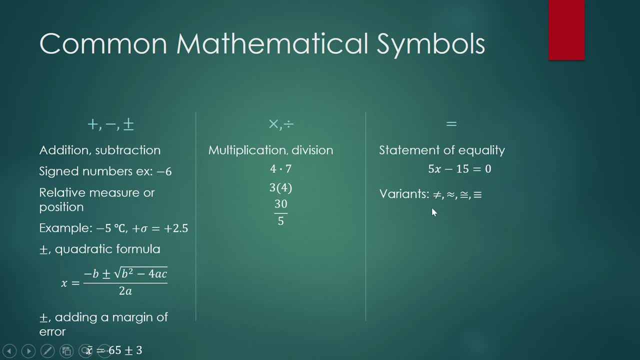 the variance of the equal sign would be not equal to approximately equal to okay. so when you're rounding off numbers with a long string of decimal numbers, so you round them off, what you come up is an approximate value and you would use this symbol for that. this one is congruence. this one means identical to congruence. 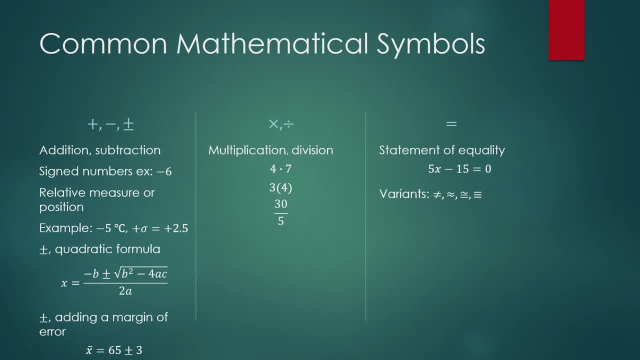 is something like this. let's say, for example, you have two triangles. you put one triangle on top of the other. if they perfectly match each other, if they perfectly fit and match each other, that means they are congruent. Less than or equal to, greater than or equal to. Example X is greater than or equal to 12. 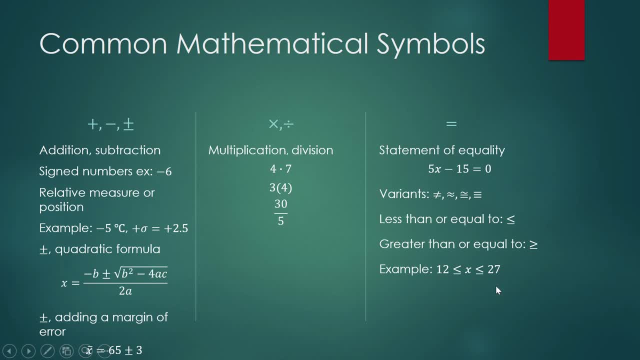 and less than or equal to 27.. So when I was a student, this was the allowable number of units student must enroll during a regular semester. Your load must be not less than 12, okay, And it should not be greater than 27.. When I was a 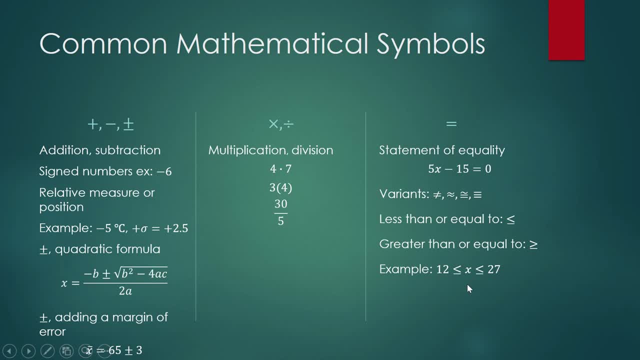 student, there were occasions wherein I would choose only to enroll in 12 units. The regular load was 18 units. So I was choosing 12 units so that I can give time to my other hobbies. you know, when I was a student, I like to run, I like to. 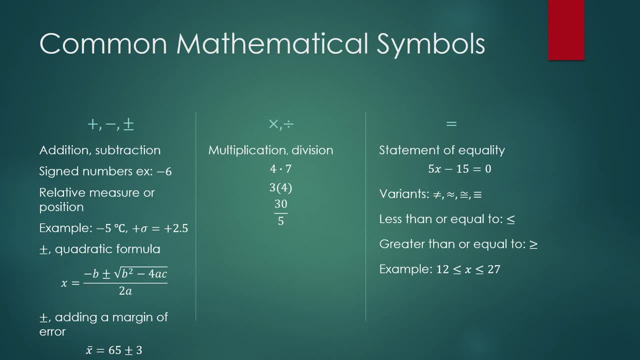 play basketball. I also trained in martial arts, so I wanted to give, I want to devote and attention to those other endeavors, which is why I was only opting to get enrolled in 15, sometimes 12 units. But you cannot get enrolled in less than 12. You will be considered an irregular student. 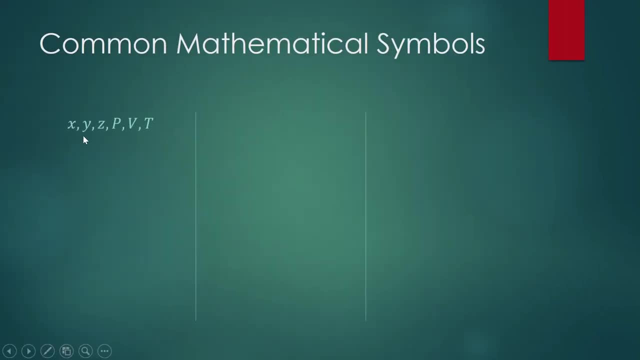 What else? So we use these symbols- small letters, capital letters- to mean variables. Okay, variables, The key word there is vary, So these are quantities that change in value. They are not constants. So P, for example, is often used as the symbol or variable for pressure, V is for volume. 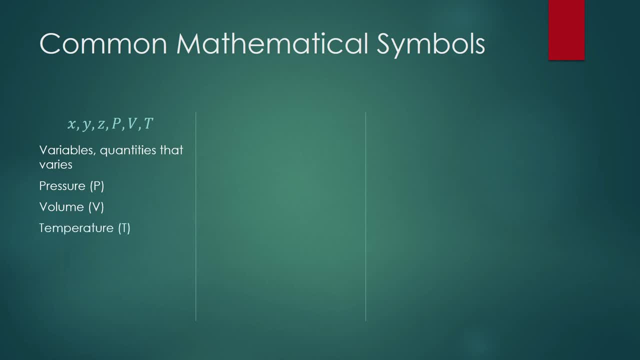 T is for temperature. You know what I can remember, my days when I was a kid and my father was still alive. It was I who was filling in butane gas into his lighter because he was smoking And it was one of my duties to fill in his lighter with butane. Butane is a gas in a 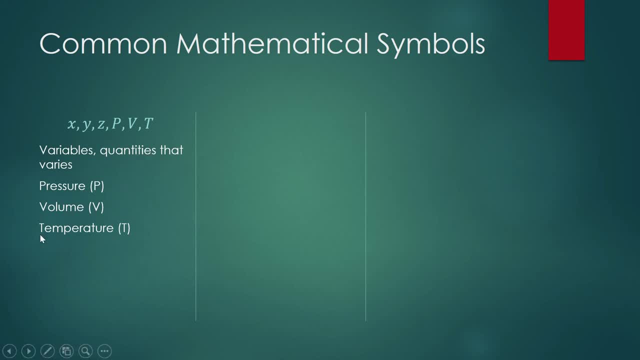 cylinder And I experienced what this means. Okay, Because when you fill in the lighter with butane gas, the gas in the container is diminished, So there is less pressure inside the tank And I can feel the temperature decreasing. The cylinder is becoming colder. 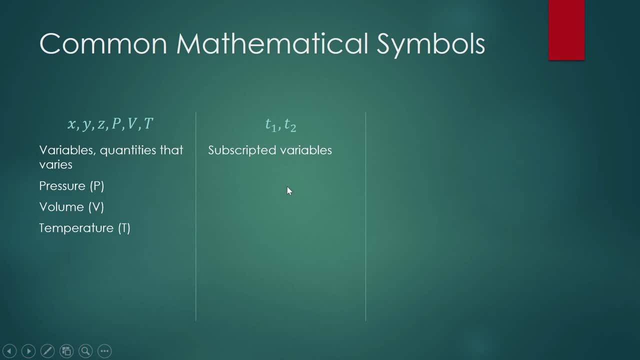 Subscripted values T1 or T2.. So T1 and T2 are subscripted variables. Subscripted, That is what you call the subscript. Okay, so what is? let's say, for example, T stands for temperature. So in: 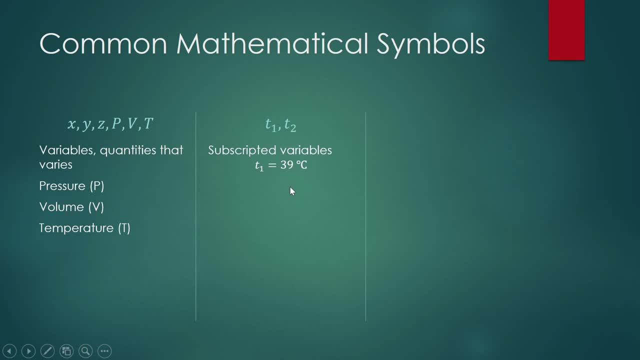 the first time you took your brother's temperature- he was sick- was 39 degrees Celsius. After two hours you took it again. You took the temperature, You measured his temperature. It was 38.1 degrees Celsius. And you took it for the third time after the passing of two more hours And it's now. 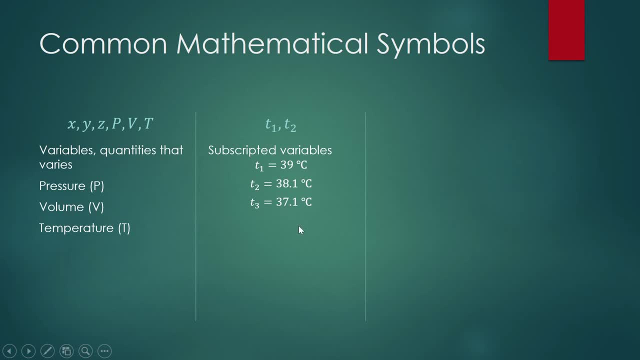 37.1 degrees Celsius. So that is how you can use these subscripted variables. Okay, so of course you are familiar with this. These are the Greek letters, small k's. We use them to name angles. We also use them as a symbol for some irrational numbers, such as. 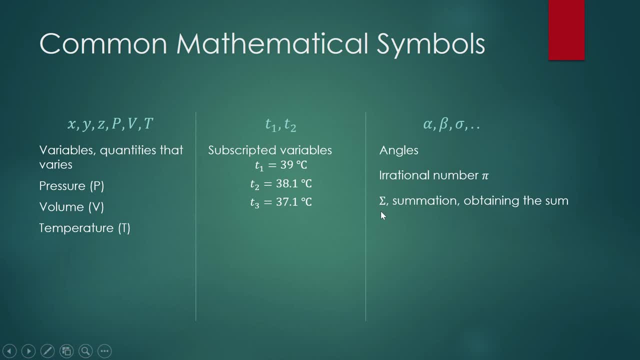 pi. This one is another Greek symbol. This is a sigma notation, but the capital letter, or the capital Greek letter for sigma. So it means summation, It means obtaining the sum. So, example, example, you have four quizzes. So you have, you would have four scores. What is the average of those four scores? So before you can get the average, you must get the sum of those four scores. 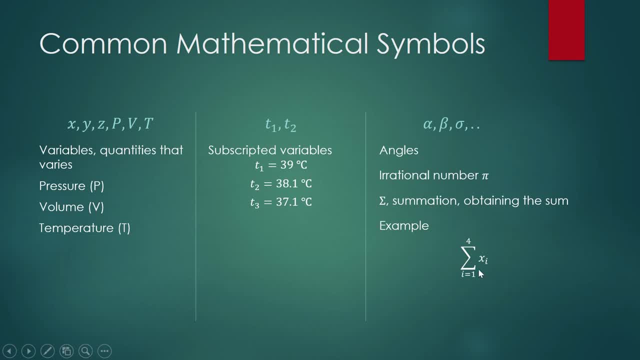 And this is how you can indicate it in math symbols: The summation of X sub i. this is how you read it: The summation of X sub i, i from 1 to 4.. And after getting the sum, you divide it by 4 to get your average score. This is pronounced as: mu mean average. You use that symbol to mean the population average. This is sigma. That is also a. 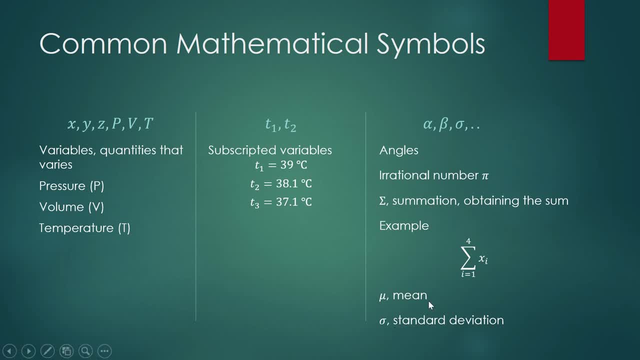 sigma notation That is also a sigma. Okay, small case of this one. So this one is used to indicate the standard deviation Square root of 9.. So square root of 25 is equal to 5, because 5 squared is equal to 25.. Fourth root- So that is how you read it- The fourth root of 16 is equal to 2.. Why? Because 2 times 2 times 2 times 2 is equal to 16.. 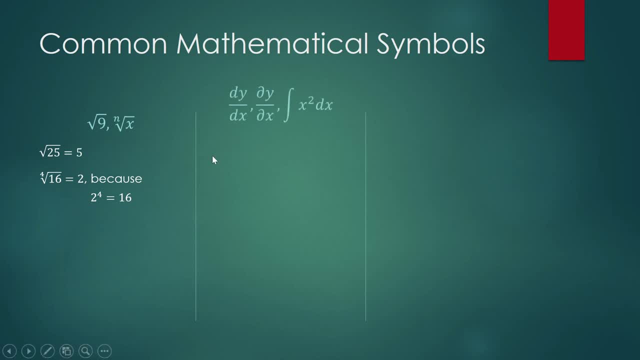 This one is probably a symbol that only STEM students saw during their high school education, And they will see this again if they were to pursue a STEM related degree in college. So dy over dx, Or this one is d sub x or dx. This is how you read it. F, prime of x, You call them derivatives. 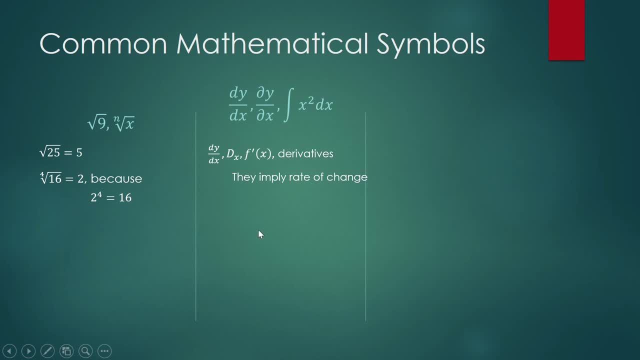 Take this up. So when you see these symbols in any book, they pertain to derivatives. All of these imply rate of change. So you should be familiar with the rate of change, Because in your junior high school math you were given the slope of a line, You were given a linear equation and your teachers told: 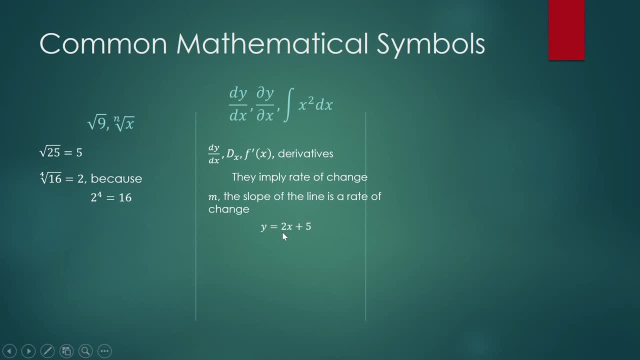 you that if your linear equation is given in this way, this is the slope of the line. And how do you get it? It's the change in Y over change in X. it is a rate of change. okay, so the slope of your line is actually a derivative. if you plan to go to higher math courses, you 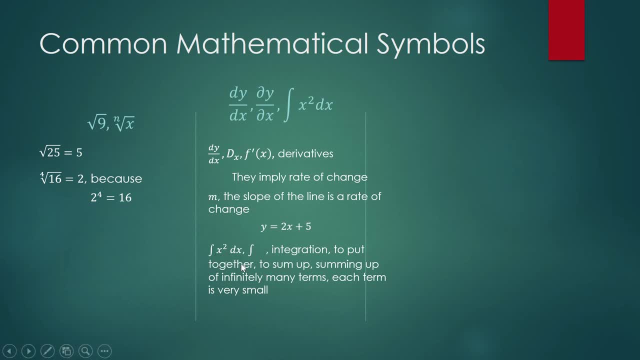 will see this: the integral of x squared DX. this symbol is called the integration symbol or the integral. okay, so what does the integration symbol imply? well, it implies the word integration. so let's say, for example, you are a group leader of a team of students who are given the task to produce a term paper, so someone 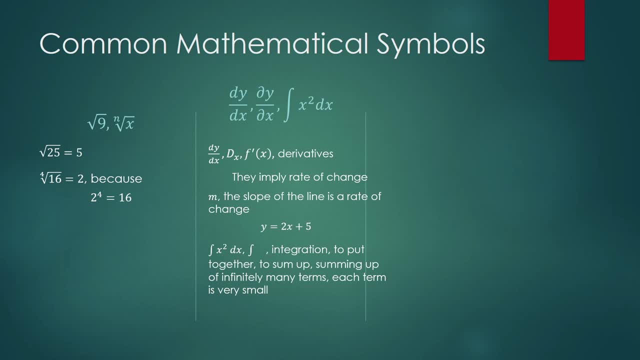 will write the introduction. someone- another one will- would write chapter one, another one would write chapter two. you will write the summary. so when you integrate all of that, you will produce a term paper, a complete term paper. so that is the meaning of integration: to put things together, but in math to put.